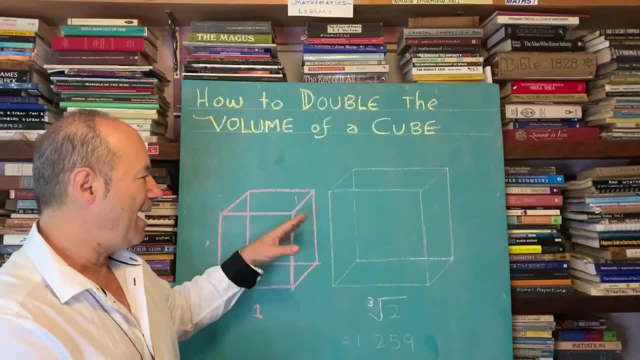 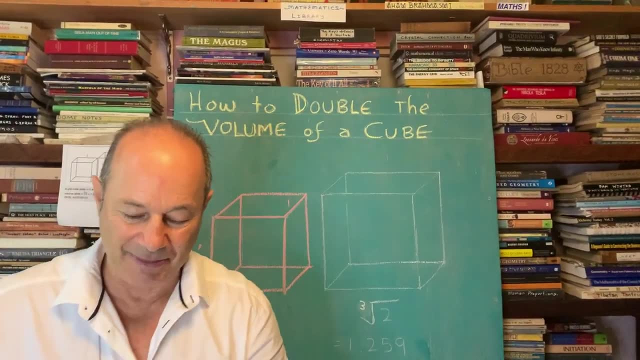 There's a very critical factor or ratio which we're coming up to- how to double the volume of the cube- And the origin of this puzzle? the origin of this puzzle comes from one of my most favourite books of all time. It's called The Secret Teachings of All Ages, by Mandy P Hall, And about 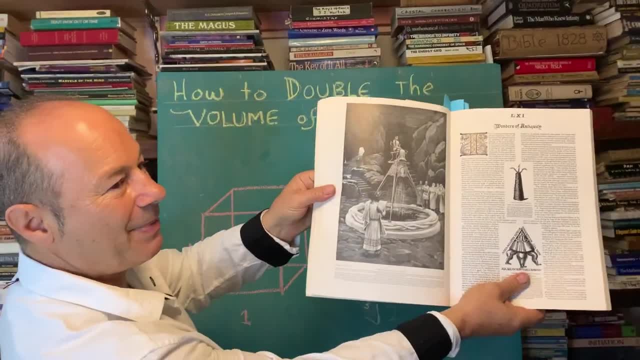 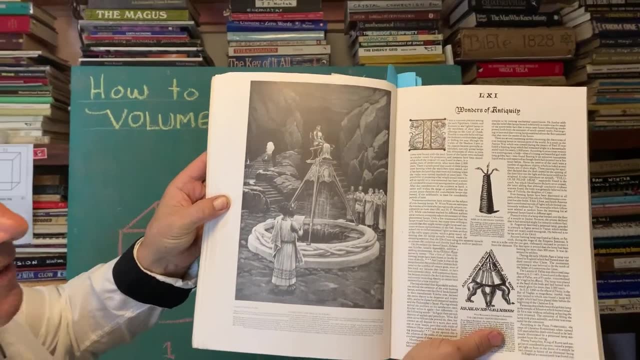 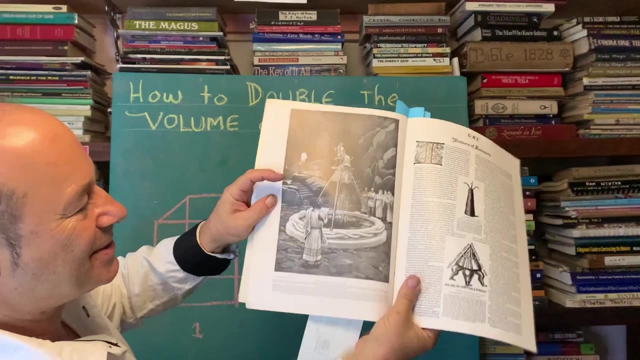 a couple of weeks ago I did a talk about the Oracle of Delphi sitting on her tetrahedron And you can see that there's kings and queens who've come. They've asked about the war: Am I going to? Am I going to win the war in France and Germany? So this is the scribe here And there's the kings. 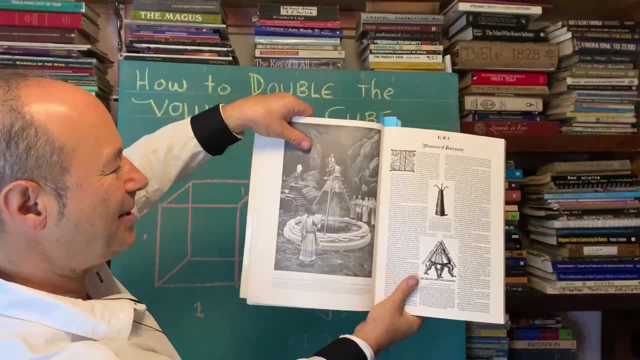 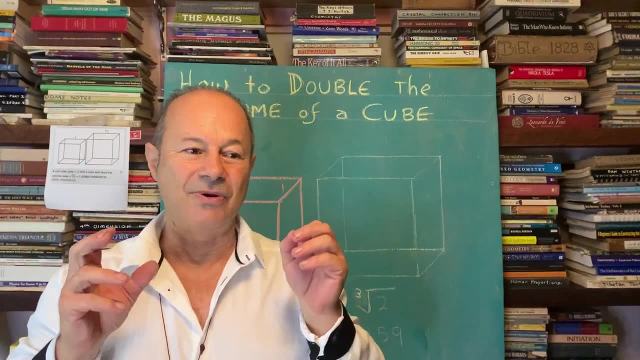 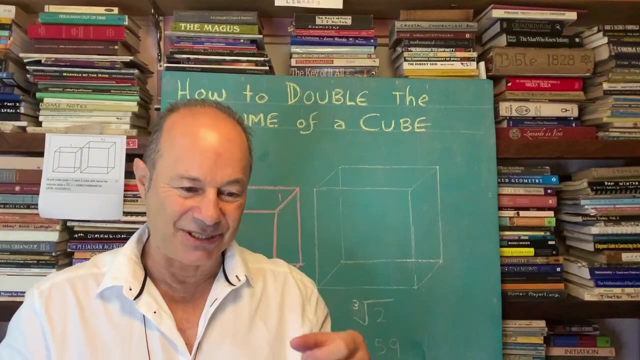 and queens and princesses consulting the Oracle. So she's going into trance and she's going and she tells them. she says, in a nutshell: to have success in your journey to win the war, I advise that you double the cube. So that was the message. They had: to divide the cube. 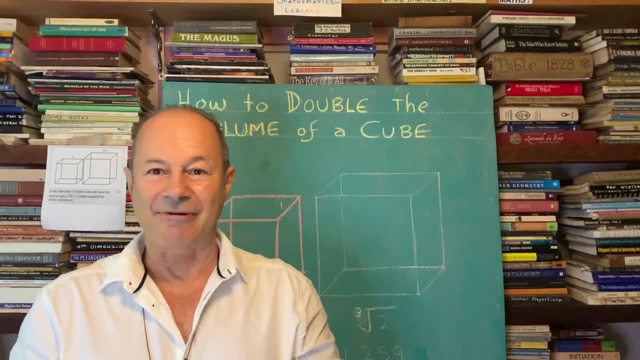 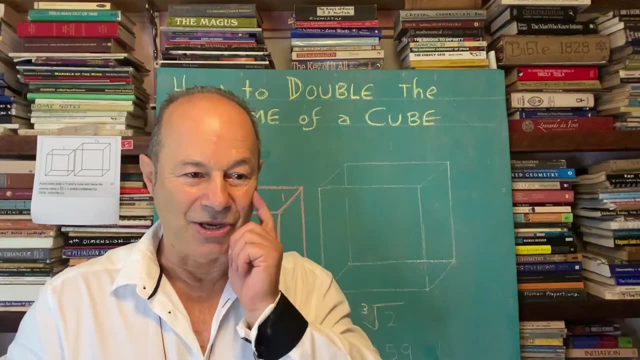 And remember this was the time- at Pythagoras And some other great mathematicians. So they went and consulted all the greatest mathematicians of the time, like you know, Euclid and that, And they said, hey, OK, what we need to do. 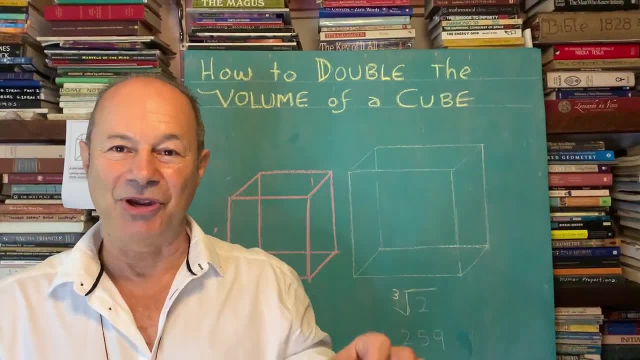 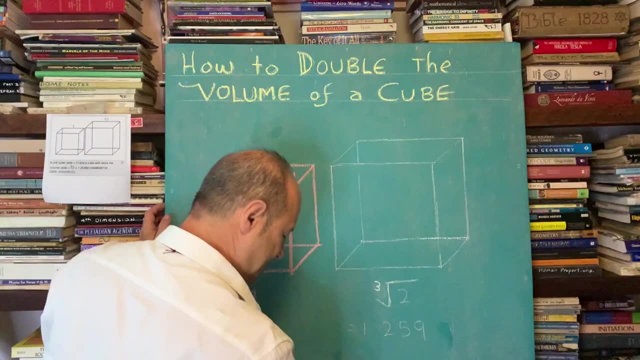 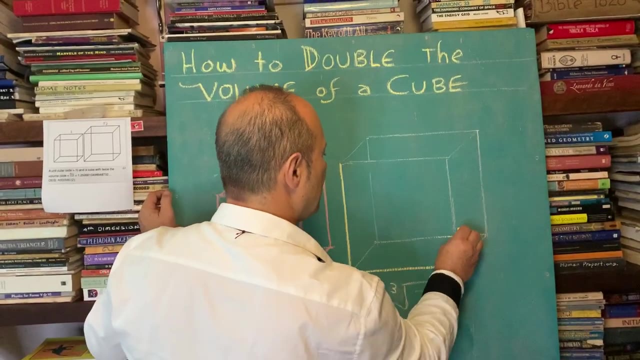 the Oracle of Delphi is asking us to double the cube literally. So this is the solution. And they did it geometrically. So the ancient Greeks did this very geometrically. The cube now is a bit bigger. We haven't worked out what it is yet, but you can see that that was a small unit cube. But now 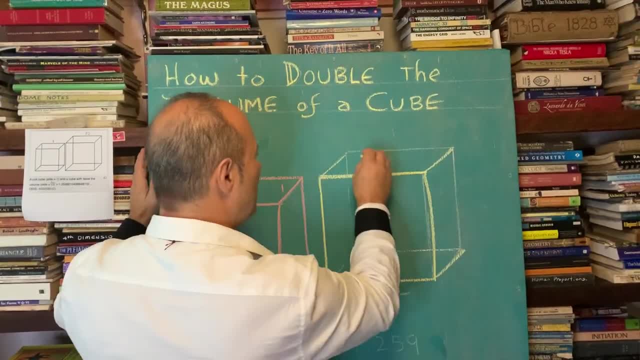 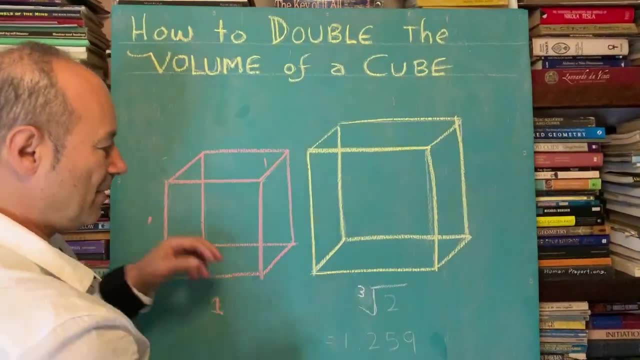 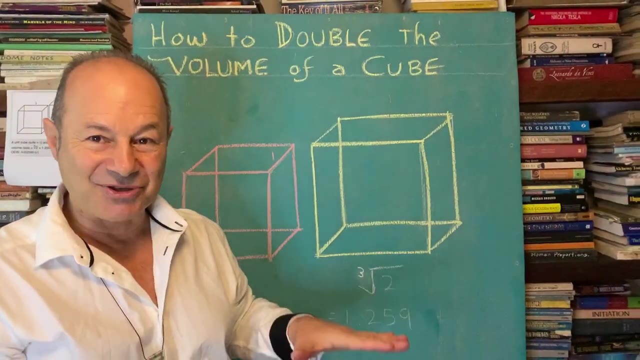 the next cube is increased. But if we were to measure the volume of this cube, we need to know the actual length. We need to know this length which is uniform And without going into all the geometry and the algebra that was required. this is like a highly intelligent question and 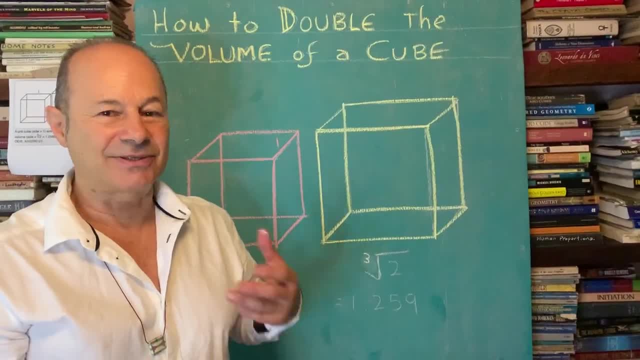 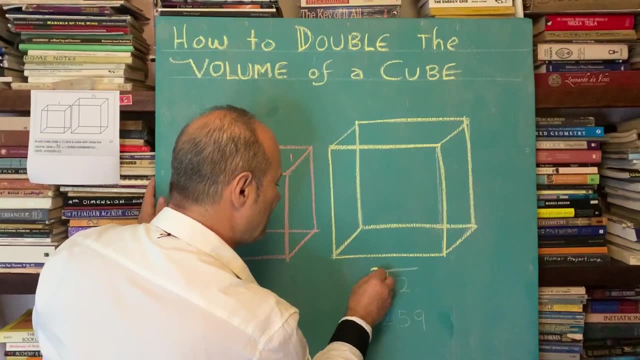 required the great mathematicians to do it, So they did it geometrically. So this is the greatest minds of our history time to get this right. So what I'm going to do is I'm going to tell you that it was based on the number two, because we're doubling, So that baby three there. 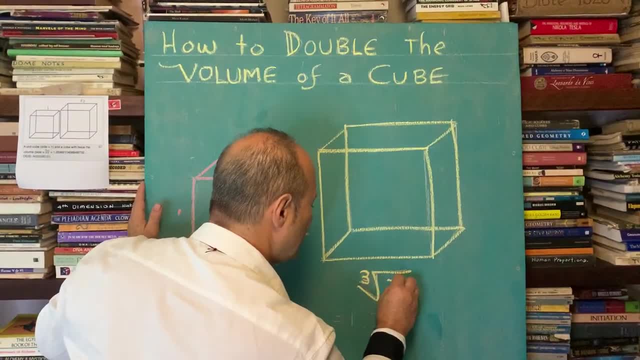 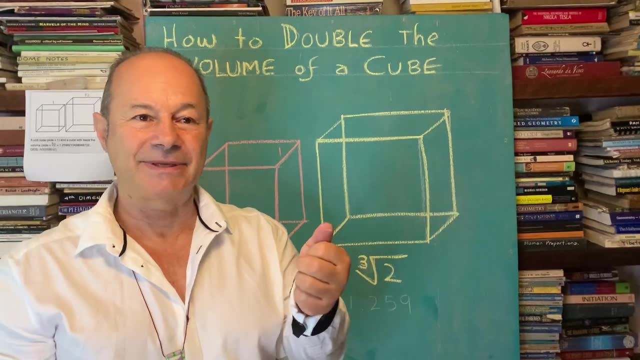 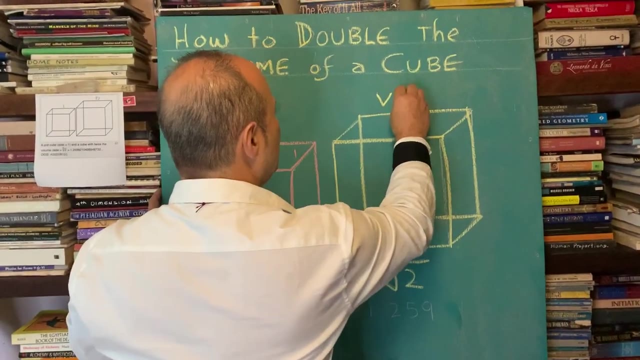 is called the cube root, So the cube root of two. that's the solution. The cube root of two means what number multiplied by itself, three times, will give two, Because this is the volume of one. But we want the volume here. So we're going to say that the cube root of three times is equal to two. So on your calculator here. 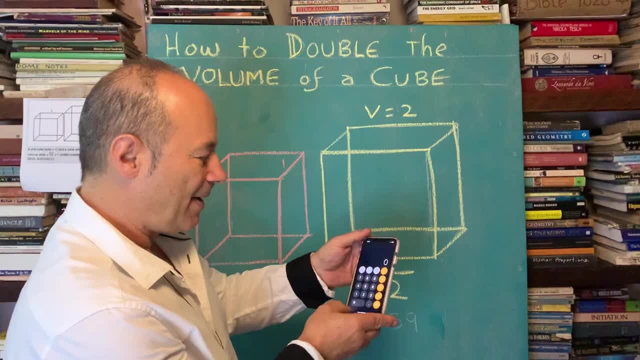 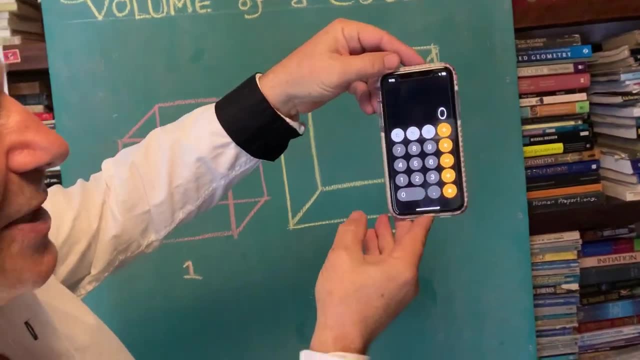 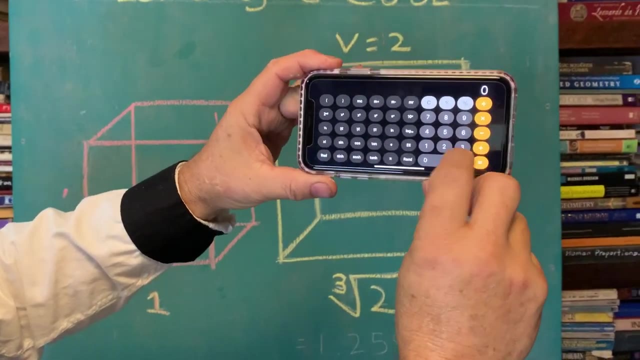 without showing you all the algebra. I have my calculator here, scientific calculator. If I turn it this way here. did you see how I went from? that's normal calculation. When I turn it like this, I end up getting a scientific calculator. So I want the number two, So there's two And I 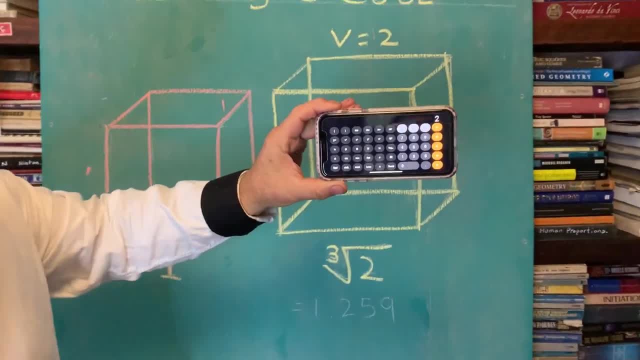 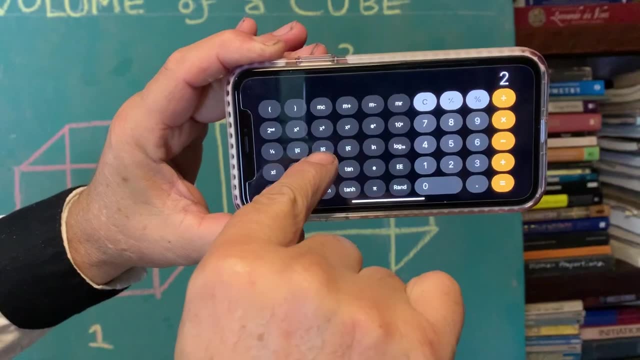 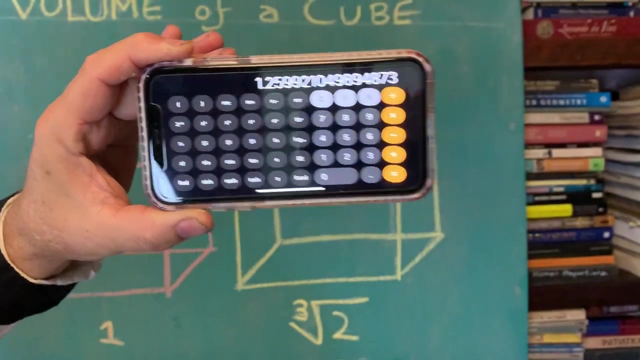 want to find the cubed root of two. So if you look closely, if you look closely at this- I'm going to touch it here- You can see an x, the cube root of x, with a little 3 there. So when I touch the x, the cubed root of 2 is 1.259.. I'm going to write that. 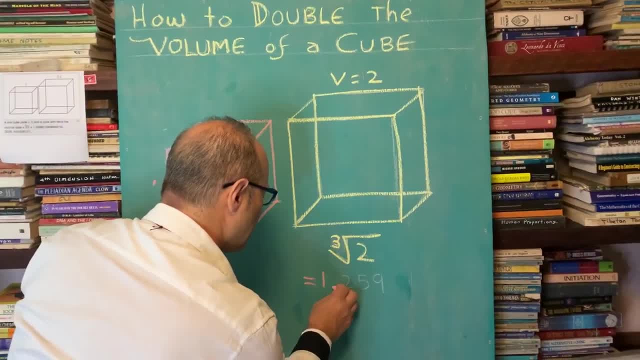 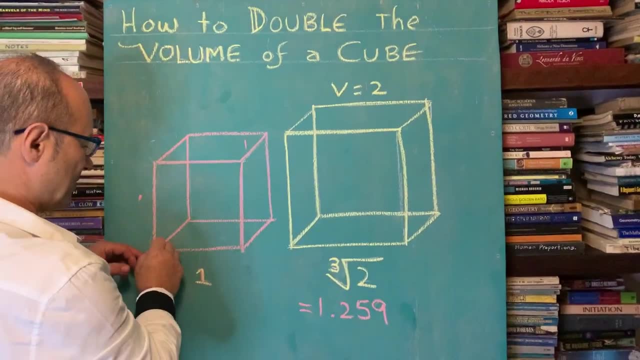 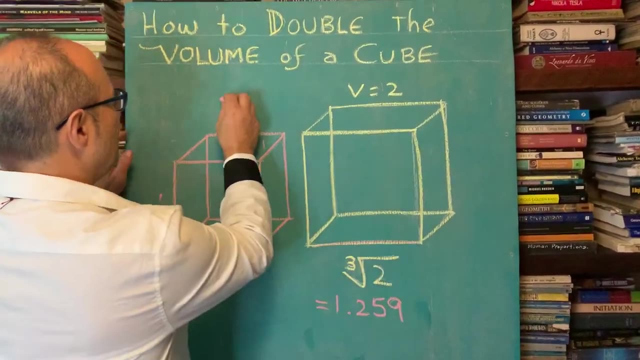 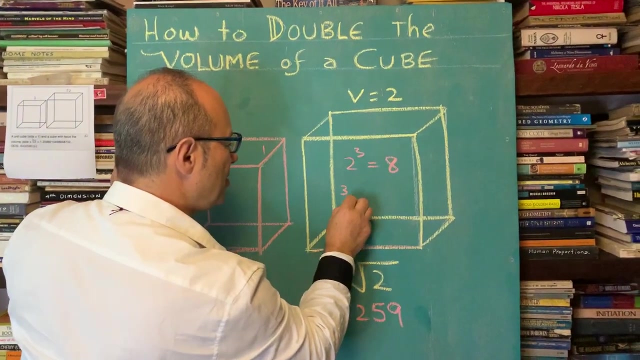 down So it equals. the answer was 1.259.. And the reason I'm saying this is that most people would say that if this is 1,, to double our cube we go a length of 2 units, But 2 cubed equals 8.. So that can't be the answer, because the cubed root of 8 means what number? 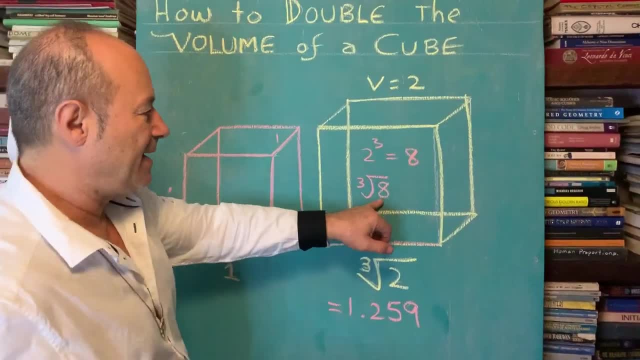 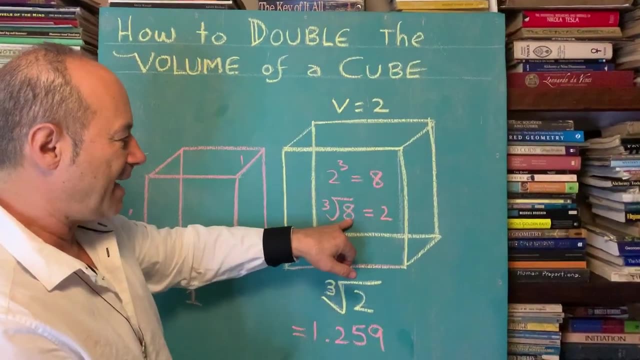 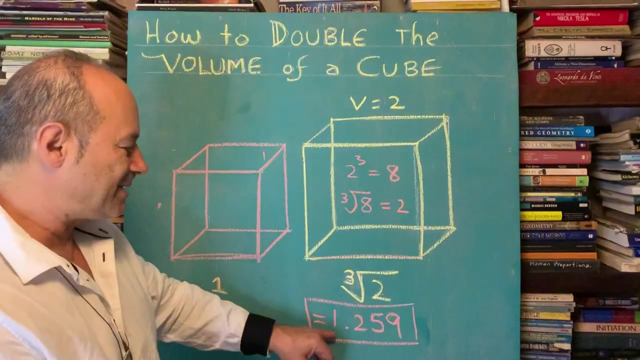 multiplied by itself gives 8.. So the cubed root of 8 is 2, because 2 times 2 times 2 equals the 8.. So you can see here that To find the cubic solution to this problem we had to know a very critical ratio: 1.259.. 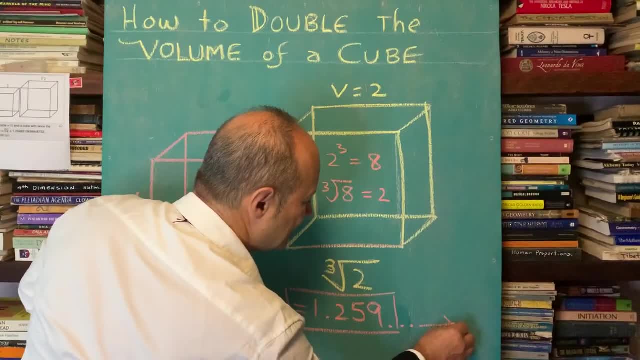 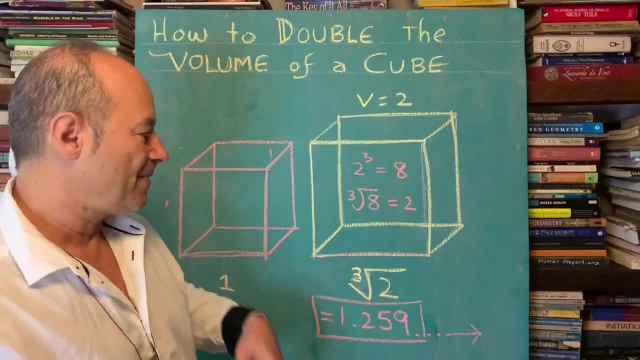 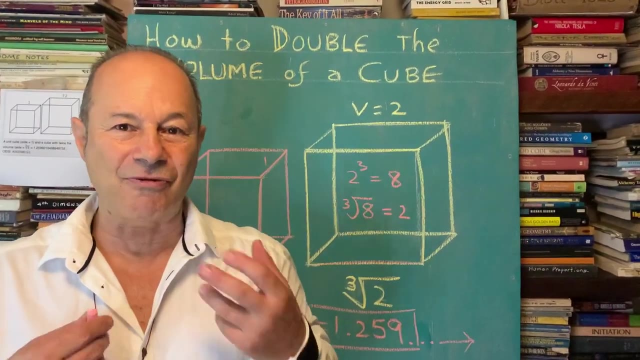 And often we put three dots after it because it means that those decimals go forever. It doesn't go: 2.2590.. It goes on and on. So I just wanted to show you that mathematicians, for thousands of years, have been completely engrossed and mystified by 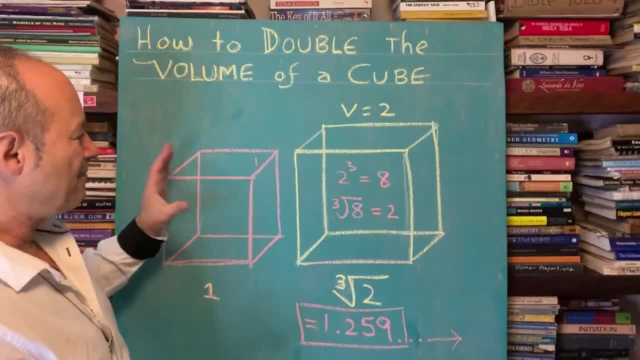 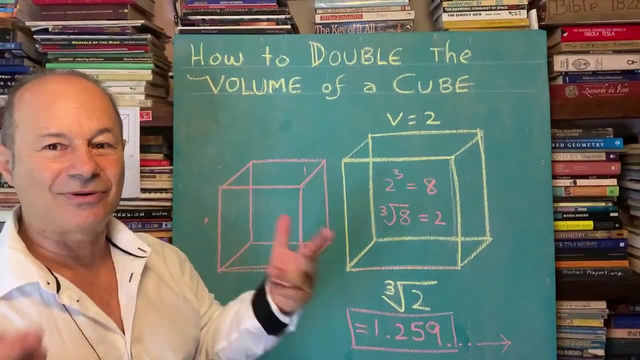 certain volumes of information, But the reason why this one is interesting is that it's in our history 2.5 thousand years ago, And it came through a channel. It came through like a priestess of knowledge, And so she knew that to win the war, we had to double.